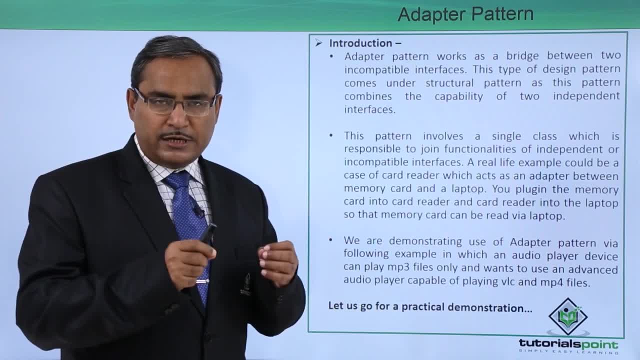 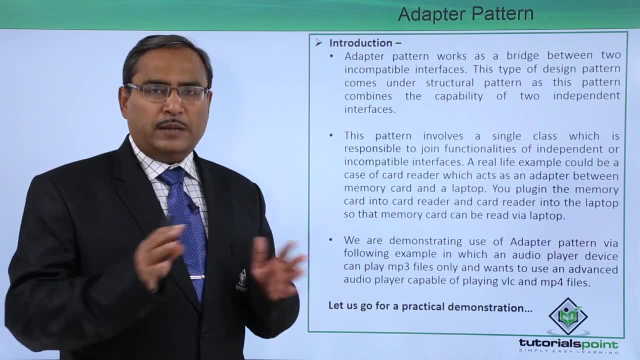 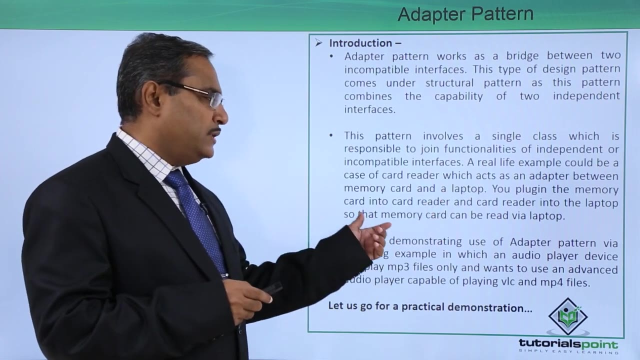 a memory card with a laptop, We require one card reader in between. So this card reader will work as a bridge between these two incompatible devices. So you plug in the memory card into card reader and card reader into the laptop so that the memory card can be read, can be written by the laptop. 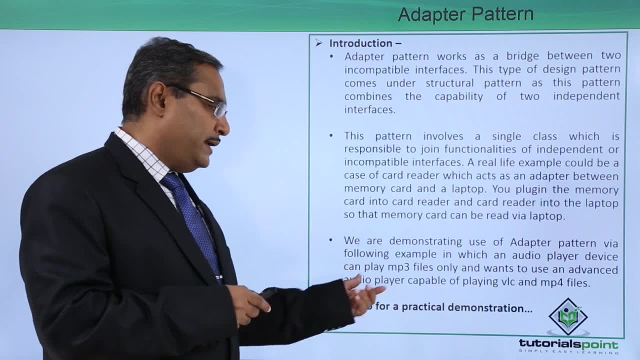 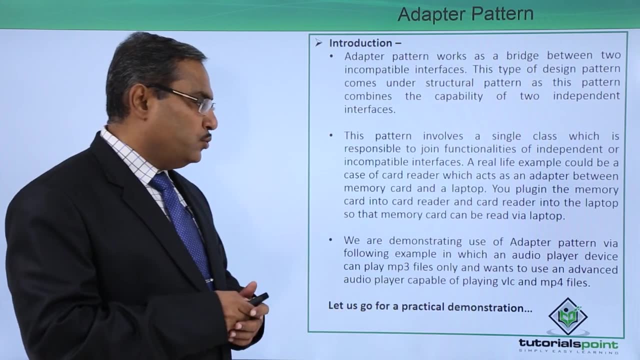 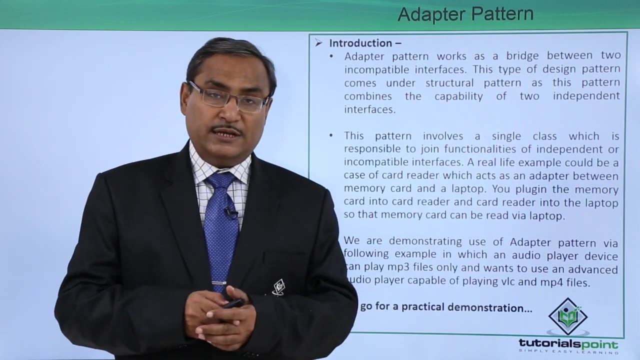 We are demonstrating the use of adapter pattern by a following example: in which an audio player device can play MP3.. The audio player can play MP3 files only and wants to use an advanced audio player capable of playing VLC and MP4 files. So I think from this the conception is not getting clear. 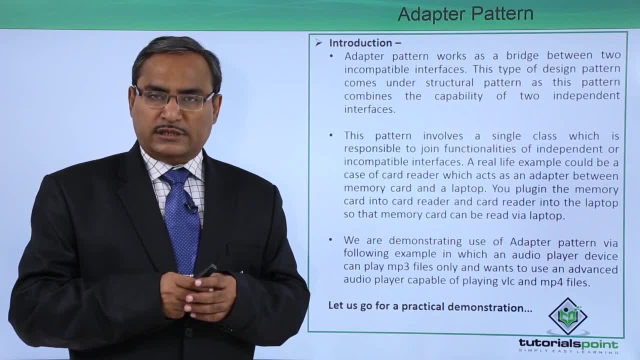 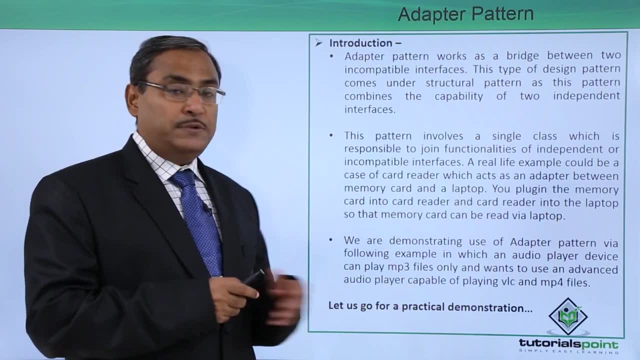 So let us go for one practical example, where we will be writing one Java application and using UML class diagrams, we shall discuss details about this adapter design pattern. So here is the demonstration for you. Now, in this demonstration, we are going to use the adapter design pattern. So here is the demonstration for you. 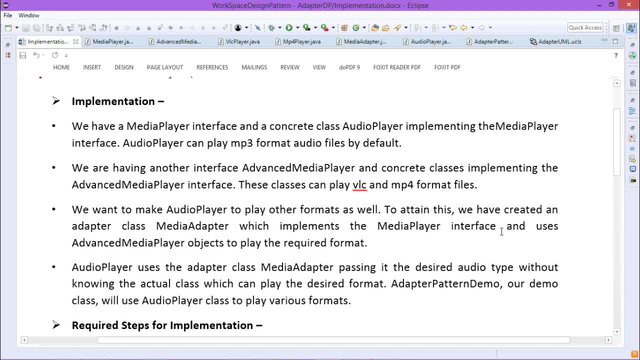 Now, in this demonstration we are going to use the adapter design pattern. So here is the demonstration for you. We are going to discuss how to implement adapter design pattern. So for the implementation, we will be considering one case study And in the case study we will be having one interface, that is the media player interface, and there is one 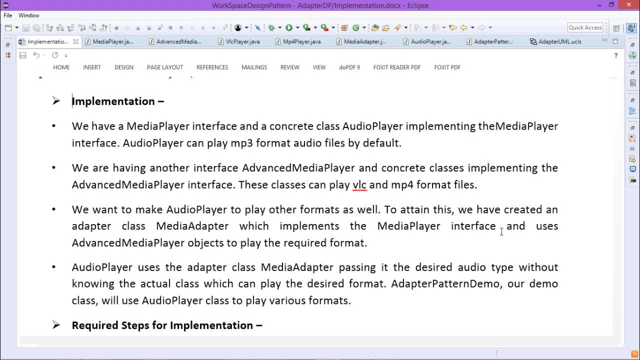 concrete class, that is, the audio player, implementing the media player interface. The audio player can play MP3 format audio files by default. We are going to have another interface. the name of the interface will be Advance Media Player and concrete classes, which will be called AMP3.. 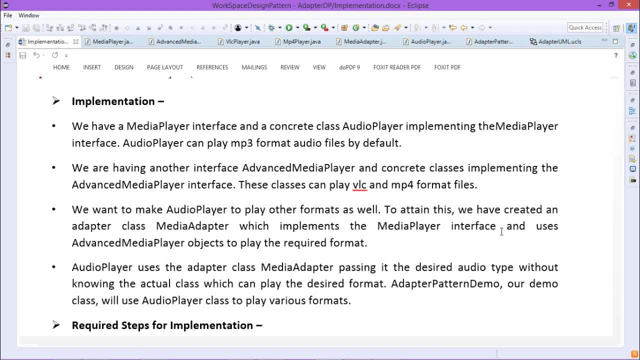 be implementing this interface, that is, the advanced media player will be having the name that is our VLC player and mp4 player, and they can play VLC and mp4 format files. we want to make audio player to play other formats as well, so that is, other formats are there, so we want to play those particular media. 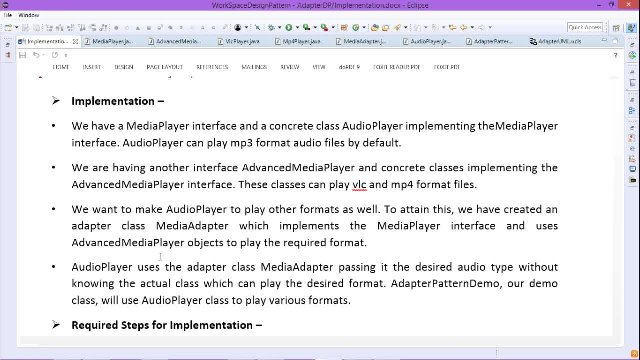 files in the audio player. so to add, to attend this, we have created an adapter class, known as a media adapter, which implements the media player interface and uses advanced media player objects to play the required format. so audio player also uses the adapter class, media adapter, passing it the desired audio. 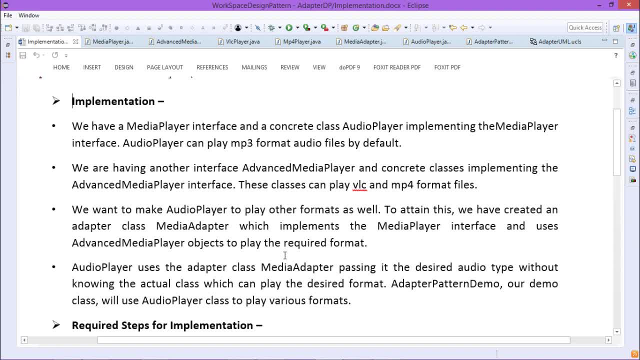 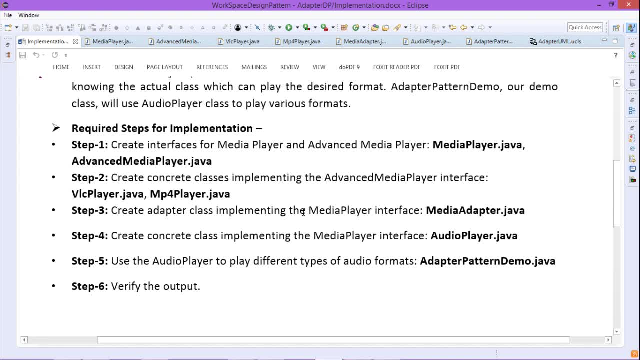 type without knowing the actual class which can play the desired format. so adapter pattern demo will be about demo class and which will use audio player class to play various different formats in the and produce the required outputs. you so to have this particular implementation we are going through 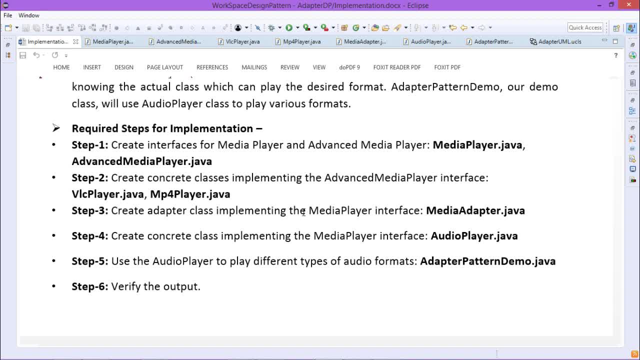 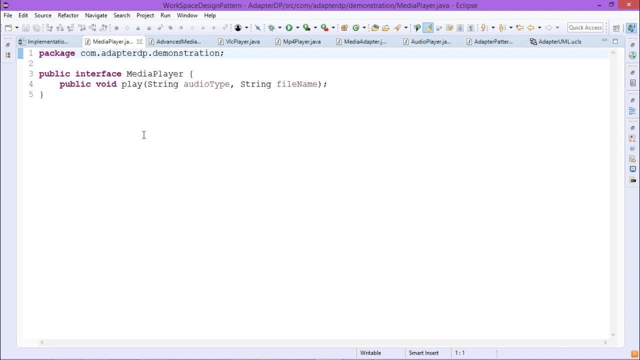 certain number of steps. so create interfaces for media player and advanced media player. so media player dot Java and advanced media player dot Java will be having our two interface files. so let me discuss them. let me show you the what to be the code for that. so public interface, media player, so media player. 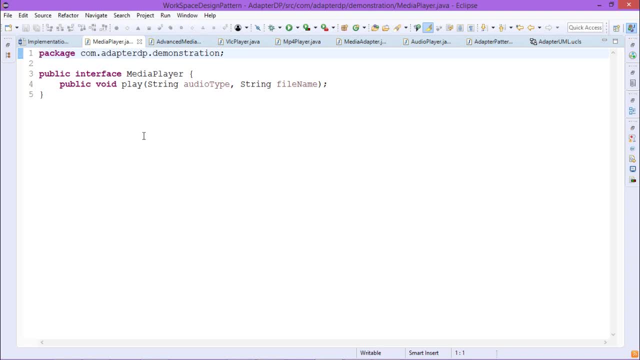 is nothing but one interface. it is having only one method, that is, a play which takes the audio type as input and file name as input. so audio type in the file name. both will be of the type of string, so string objects, so they'll be taken as input and the name of the 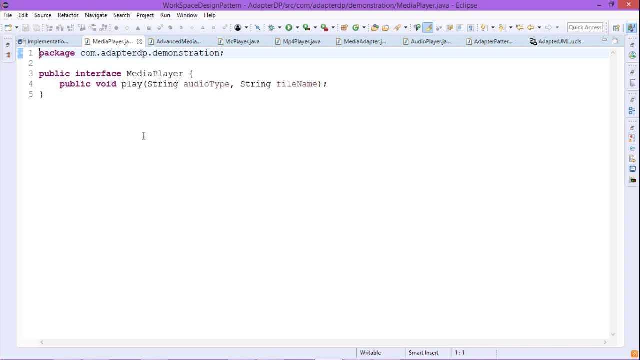 method is play, which returns what. so here this interface name is media player. so now let us go for the advanced media player interface. so instead of play here, where having play Girls It and Play mp4? so here we are passing only one input document, that is a string file name. 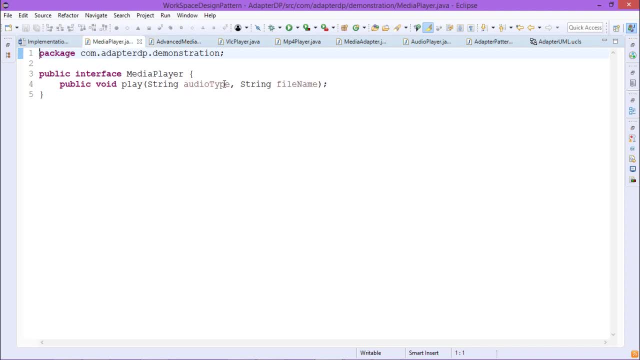 object. in the initial case i have passed this audio type and the file name, but here, as from the very particular method name, pill play vlc. so it indicates that it will. it can play only the vlc media files, and next one is the play mp4, which plays only the mp4 media file. so here we are not. 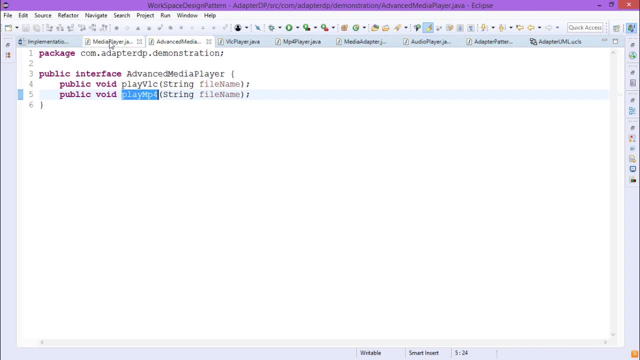 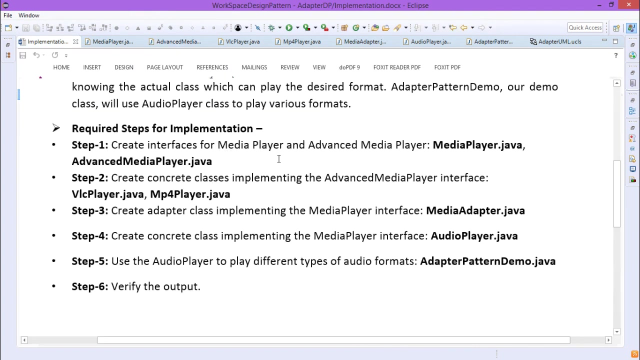 passing the type, we are passing only the file name. so we have defined this play media player. so there is a media player, one interface, and here we have defined one advanced media player, another interface. so we have covered the step number one. so next one: create concrete classes. 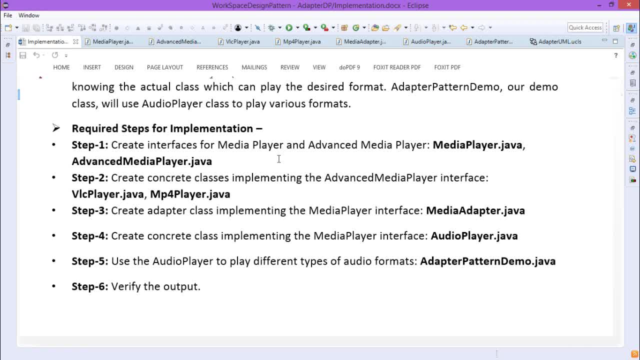 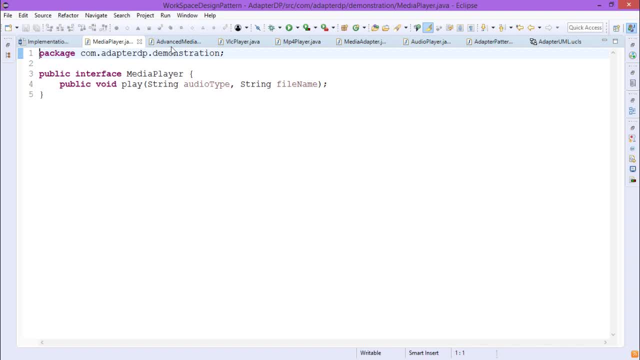 implementing the advanced media plate interface and they will be vlc player dot java and mp4 player dot java. so this is our media player interface we have discussed earlier. this is our advanced media player interface. so now i'm going to implement this advanced media plate interface in certain classes. the name of the class will be vlc player and mp4 player dot java. 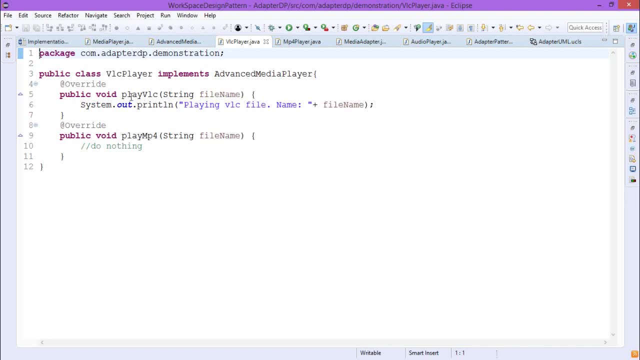 so class player implements advanced media player, so so play vlc. this particular method is going to get overwritten here, so it is. it is taking the file name as a string object, as input parameter, so we are printing this respective line. so playing with a vlc file and the name is concatenation. 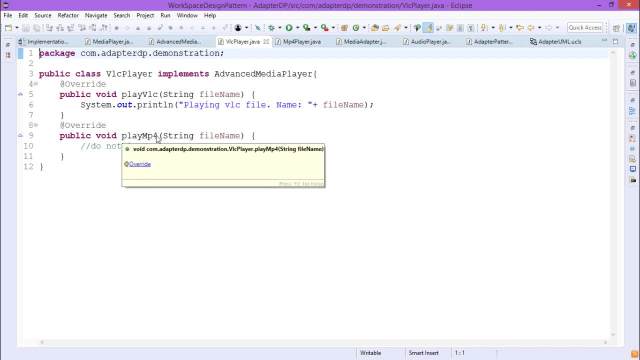 file name and this is about a play mp4 for this particular vlc player class. for this play mp4 method, we are just overwriting and writing no code there. actually, this is just the opening curly braces and the closing curly braces we are having. so next we are having this mp4 player. 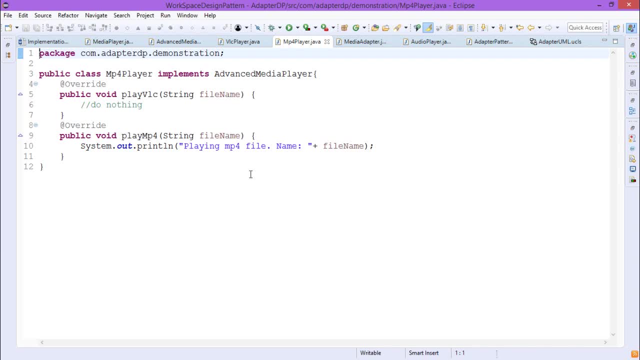 so it is also implementing the advanced media player interface. and here you see, in case of play vlc method, we are writing nothing, but in case of play mp4 method, we are just printing this respective statement there. so that is about mp4 player. so vlc player and mp4 player. 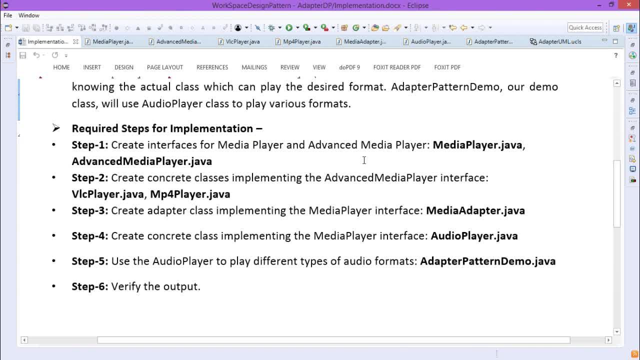 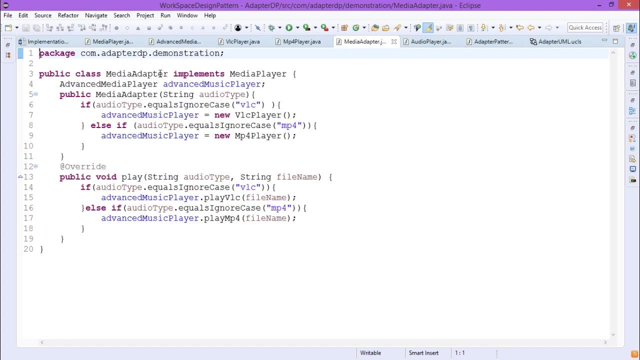 so we have covered, we have. we have discussed step number two. so now we are going for the create adapter class implementation. so let us go for the media adapterjava. so, as we discuss that media adapterjava, this particular media adapter class will implement the media player interface. so we know that in case of 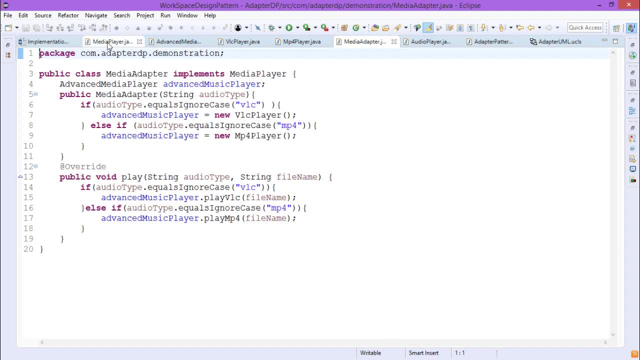 media player interface. we are having only one method defined. that is our play. so only one method is defined. that is our play. so we are going to go for the media adapterjava. so we are going to go for the media adapterjava. so this is the media adapter, this is the constructor. 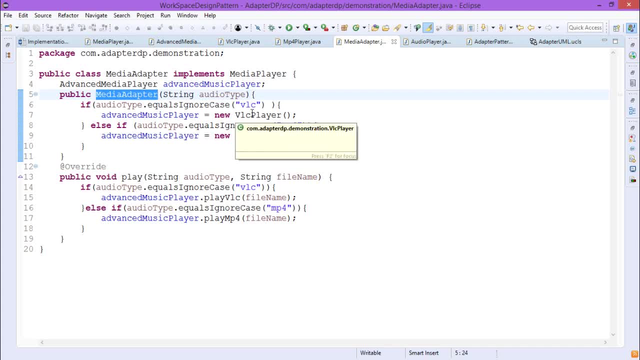 you can find that this is a constructor is a parameterized constructor which takes the audio type of the type of string object as input parameter. so audio type dot equals ignore case. if the, if the input parameter is vlc, then advanced music player is equal to new. 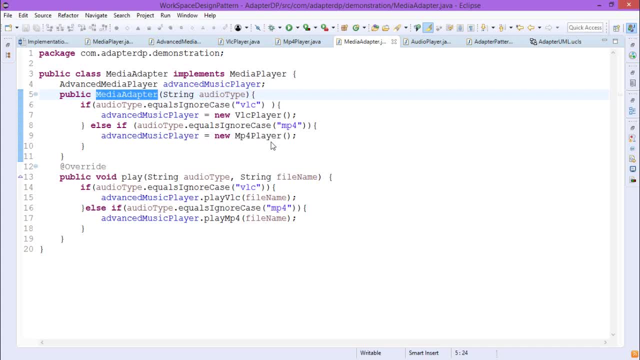 vlc player, you can find that this advanced music player is nothing but one interface. you can easily get them and this is for here. we are just, and this- this is a vlc player- is nothing but the implementing class of this advanced media player interface. so that's. 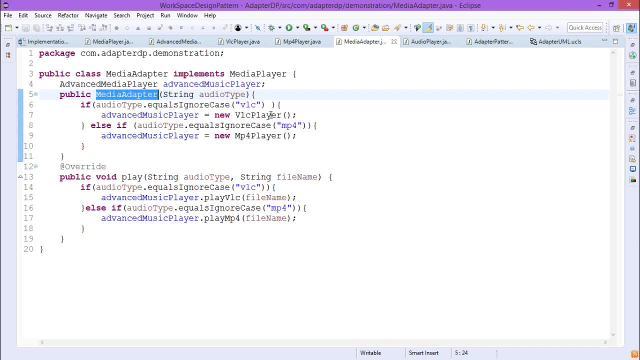 why we can easily write: advanced music player is equal to new vlc player. this advanced music player is nothing but advanced media player. interface object: okay. else if audio type dot equals, ignore case. if it, if the string is mp4, then we are just creating one mp4 player. 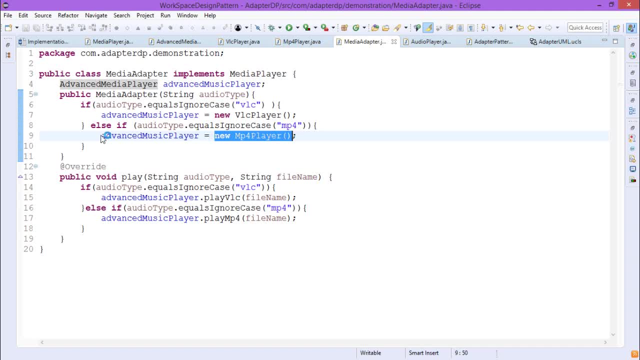 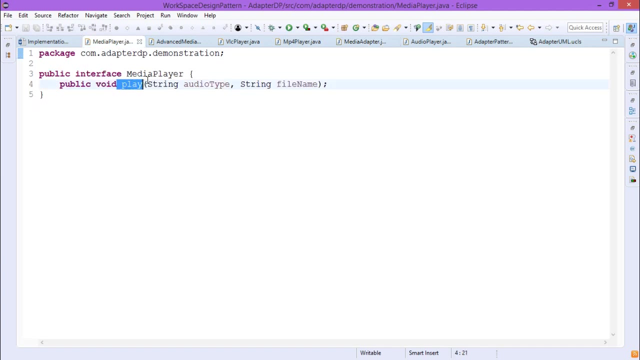 class object using this constructor, and that will be that will be taken in advanced media player, which is nothing but advanced media player interface object, as this particular class, that is, a media adapter, is implementing media player interface, so it must be writing the code for the method play. so this is a play method, so it is taking the audio type. 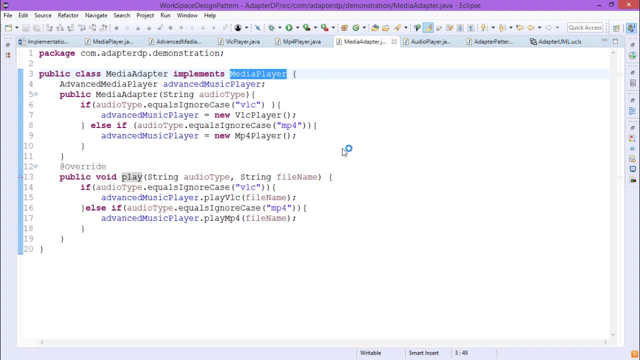 and the file name as input argument. so audio type dot equals ignore case vlc. so music advanced music player dot play vlc file name. else, if audio type dot equals ignore case mp4, then this is the advanced music player dot mp4 file name. so in this way the respective play. 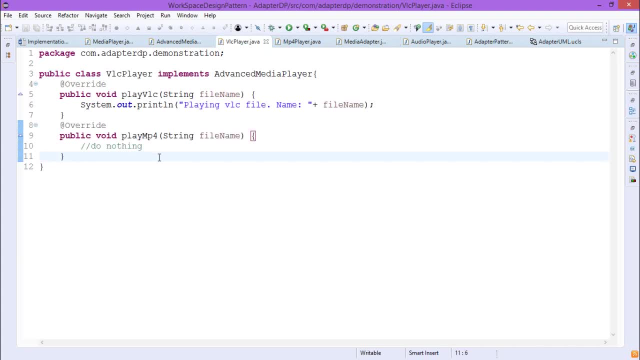 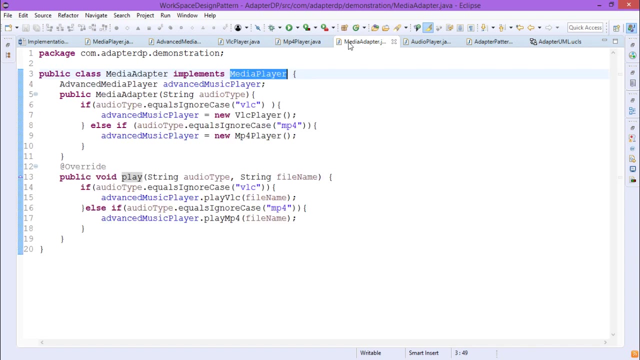 vlc. play vlc will get executed. so this is the respective code which will be executed here. and in this case, we are having this one as play mp4, so this respective code will be printed there. this respective statement will be printed. so now we are going to have this. 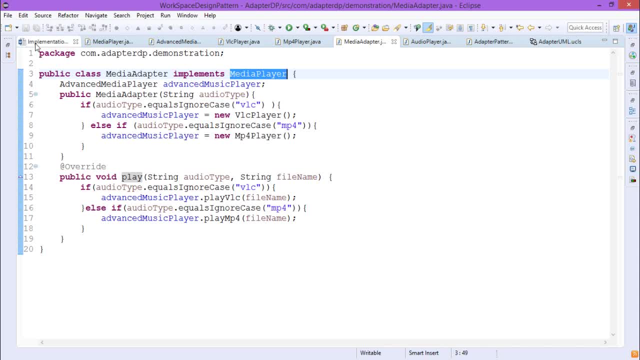 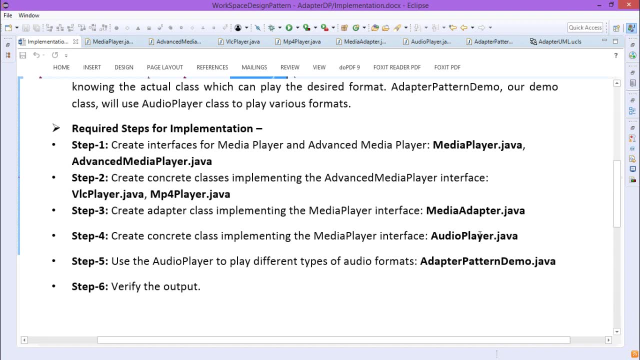 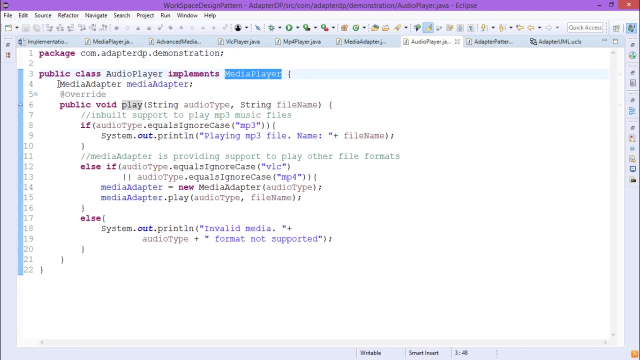 media player- media adapter. we have gone for the detailed discussion. next one we are having this: create concrete class implementing the media player interface, that is, the audio player dot java. so we are going for this audio player which is also implementing the media player. so it is taking this media adapter object as instance variable. so you know that. 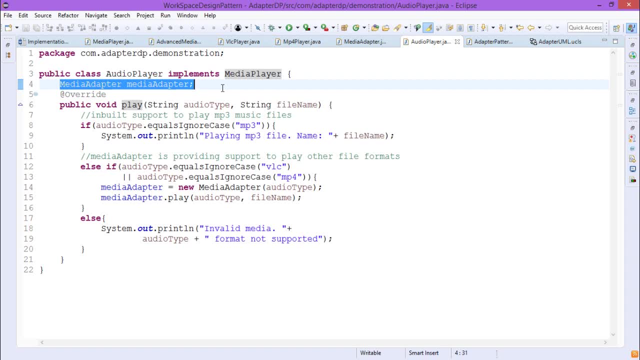 in case of media player, we are having one unimplemented method, that is a play which takes the string audio type and string file name as input parameters. so now, if audio type dot equals ignore case mp3, then system playing mp3 files name colon plus file name. so concatenation is taking place. else, if 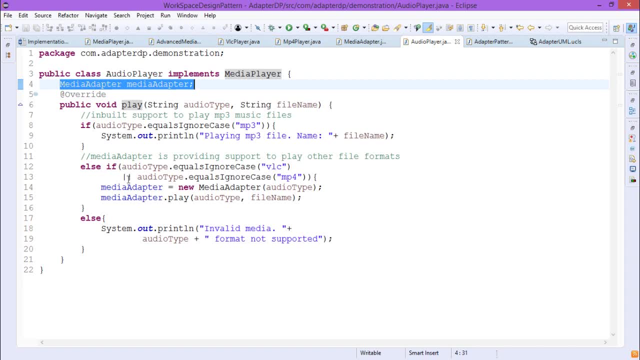 audio type dot equals, ignore case vlc. or audio type dot equals ignore case mp4, then media player is equal to new media player, audio type. now, when you are passing this uh, a vlc or this mp4 as input argument, as audio type, then the respective objects will get created and that will be, and that will be. 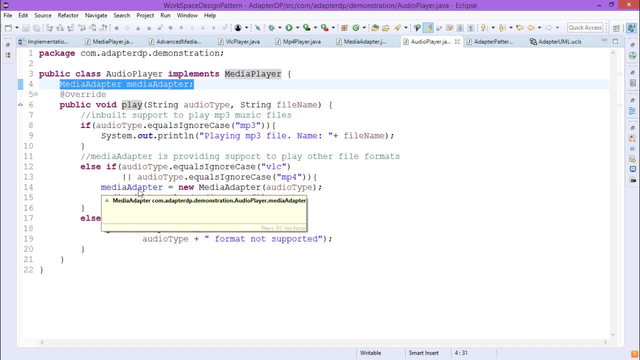 put under in this media player, media adapter, which is nothing but media adapter class object, then media adapter dot play audio type, comma, file name. so it will. it will print the respective statement on the screen, respective string on the screen. else system dot outer printl in invalid. 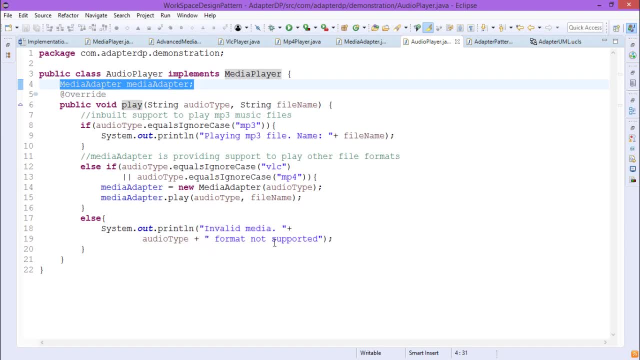 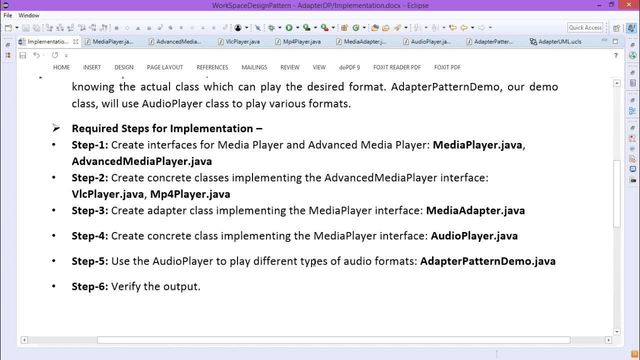 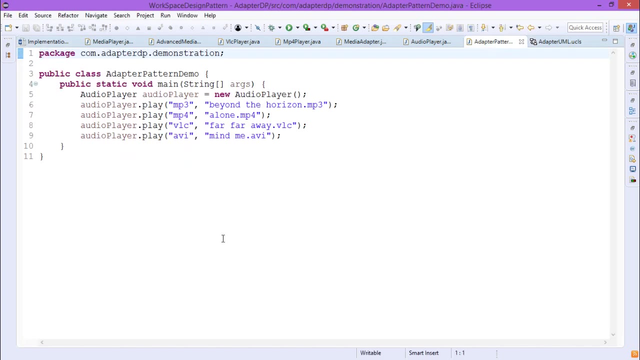 media audio type. we are getting this one concatenated format not supported. we are going to have the last class, that is, the use the audio player to play dms- different types of audio formats. that is the adapter pattern, demo dot java. so this is our adapter pattern demo dot java class. here we are having the main method. so here you have defined. 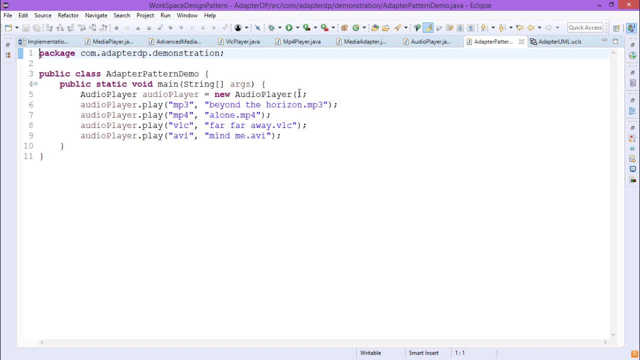 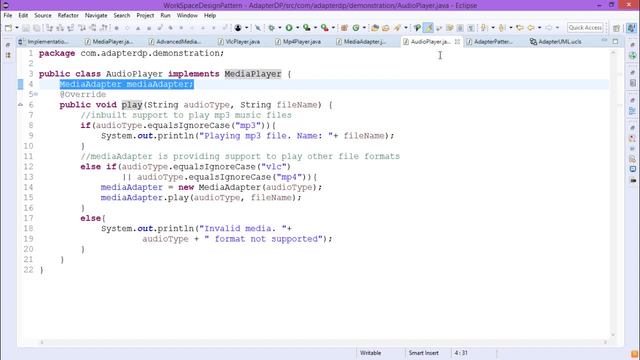 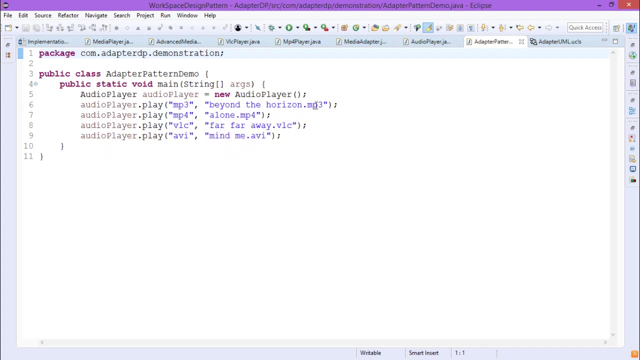 audio player class object is equal to new audio player. so this audio player class object we have defined here, so it is implementing this media plane interface. so play method is there. so now what will happen if you go for audio player dot play? mp3 is a type beyond the horizon dot mp3. 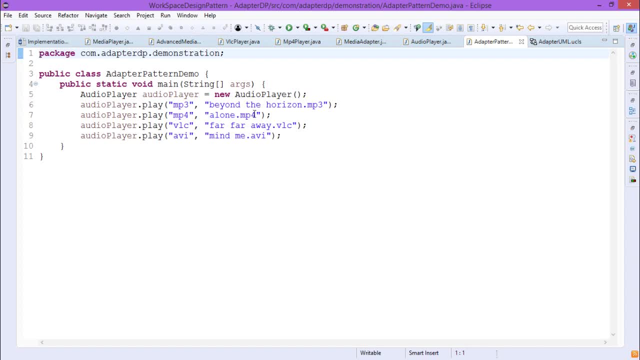 name mp4 is a type, then alone, dot mp4 is a file name in this we are having. so for this avi, obviously it is incompatible, uh, media type. so we are going to have the respective message that is format not supported. so now let me execute my code and see what outputs we are getting. so these outputs we 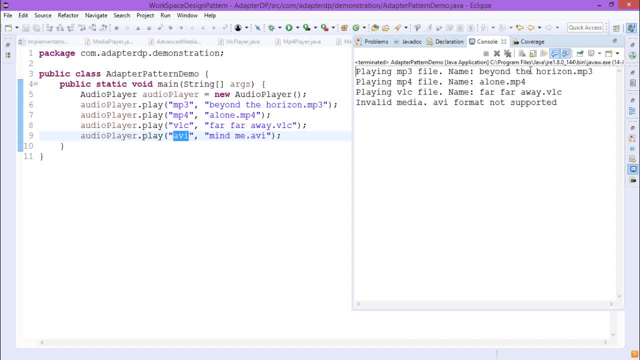 are getting, so playing mp3. file name: colon beyond the horizon dot. mp3. so there is a file name we are having here. so similarly the other outputs we are getting, and the last one is very interesting as this mp3 mp4- and we'll see only three formats: media file formats are supported. 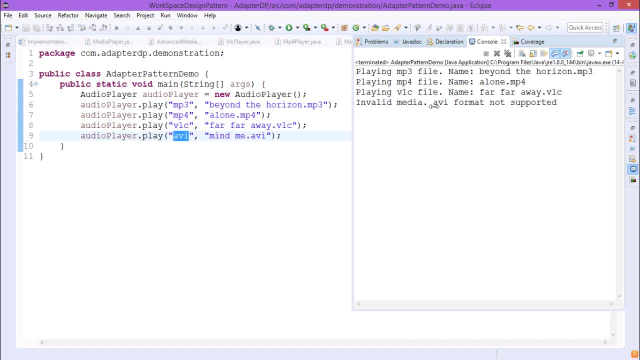 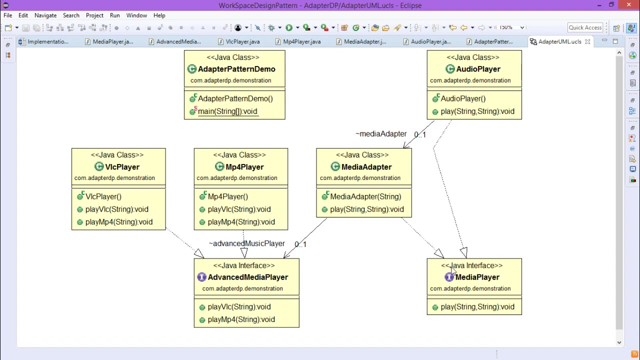 avi format is not supported here, so invalid media: uh. avi format not supported, so that message is getting printed. so this is the implementation of our adapter design pattern. so let us go for the class diagram here, email diagram we are going to have. so here we are having one java interface that